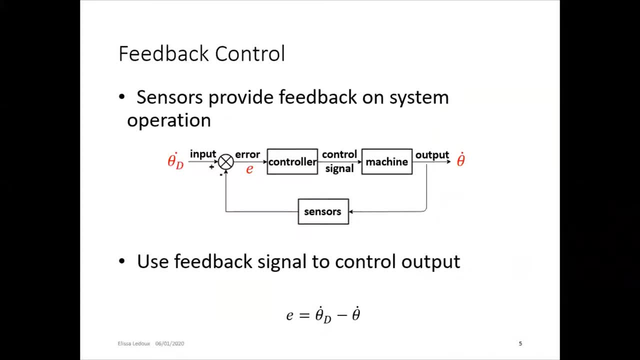 Sensors provide feedback on the system operation. You can use that feedback signal to control the output. So in a normal feedback control system you have the input, which, let's say, if this is for a motor, then you have desired motor speed. So that would be the input, And then the error signal, which is the. 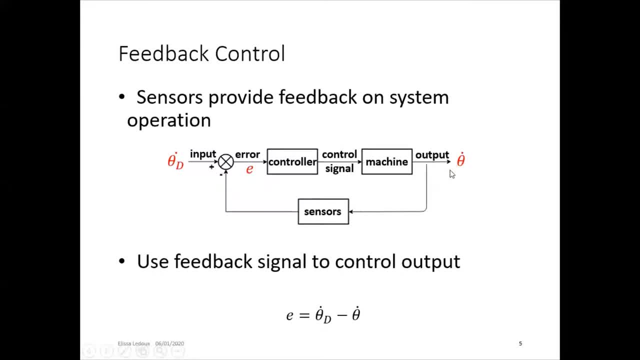 desired speed minus the actual speed. So errors: desired minus actual. So you subtract the input from the output. That's the error and the controller can work on the error. So this is a closed-loop feedback system. If you did not have sensor feedback then you would only be going based off of the input. 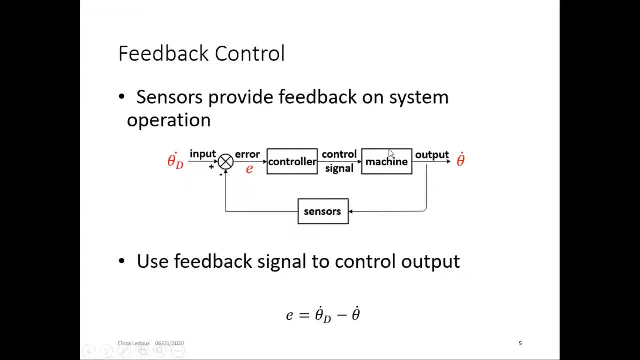 position whatever you desired. You wouldn't actually know where the system was, So the sensors closed the loop with feedback, so you can control the system based on actually what: how far away it is from where it should be based on just what you want it. 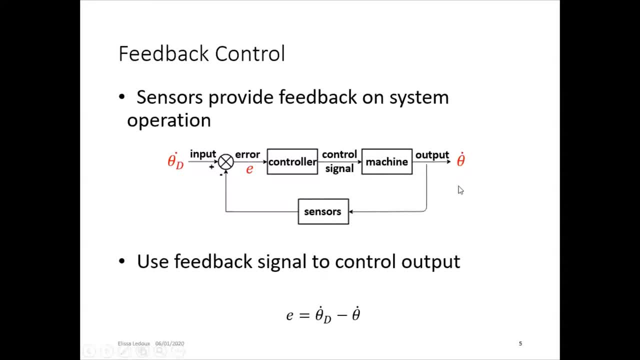 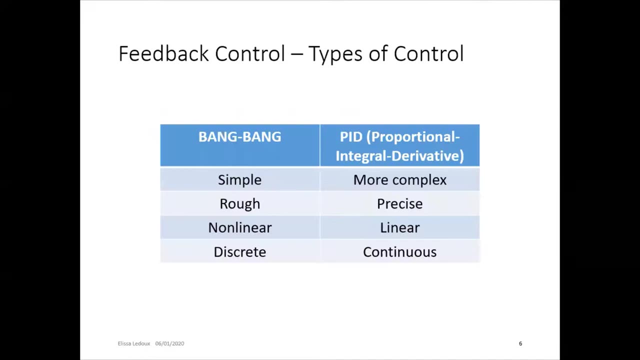 to do, And there's actually. if you're interested in learning more about feedback control, then on the ET4860 YouTube channel there are actually a whole series of videos about this type of control. But there, anyway, there are two main types of feedback control: Bang-bang. 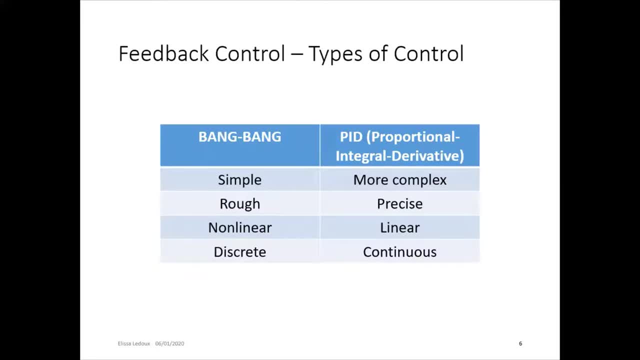 control and PID. So bang-bang control is super easy to implement. It's simple, rough, nonlinear and discrete. We'll talk about each one of these subsequently. PID control is a little more complicated, but it's a lot more precise and it is it acts. 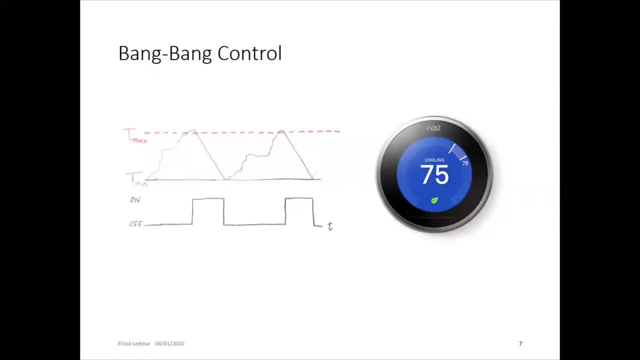 continuously. So bang-bang. control is like a thermostat: There is an upper limit and a lower limit. There is no control signal going to the system while the measure variable is in between the limits. So you can see here like temperature of the room is rising. so it's cold, the room starts to heat up. 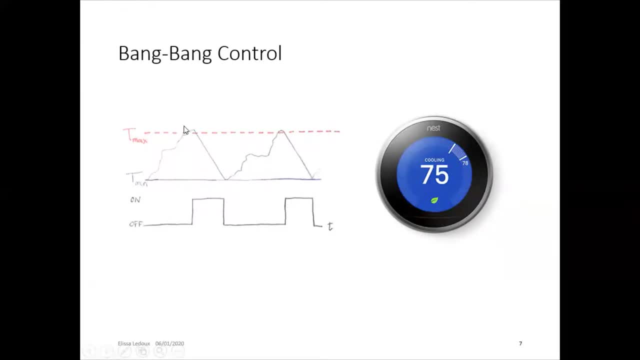 then, once it passes maximum temperature, the AC kicks on until it drives the temperature back down to the allowed minimum. Then it shuts off. Slowly the temperature comes back up again. AC kicks on, drives it back down. So you can see it's off, on, off, on. So this is why it's called bang-bang control, because when it hits the top, 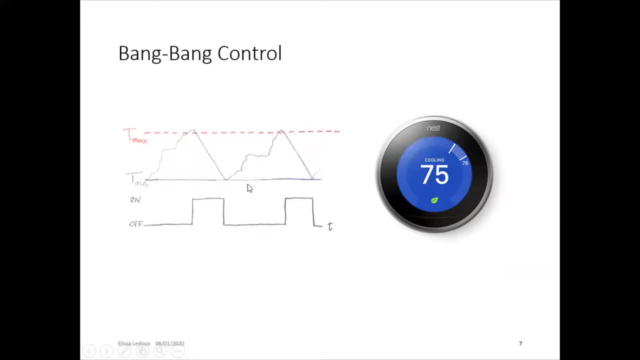 limit. it bangs it down When it hits the bottom limit, then it's also a limit. So this is super easy to implement, but also it's not very precise, because you just know that you're not keeping temperature at a certain value, you're keeping it within a range. So that would be like here: 75 to 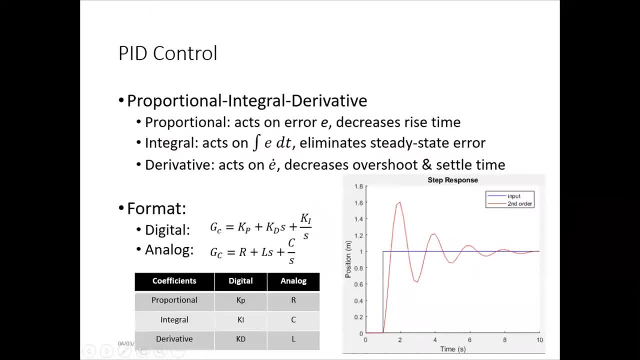 78.. The ID control is proportional integral derivative. The proportional integral derivative is the proportion of the temperature at a certain value. The proportion of the temperature at a certain value is the proportion of the temperature at a certain value, The proportional constant AP. that acts on the error and it decreases the rise time. So 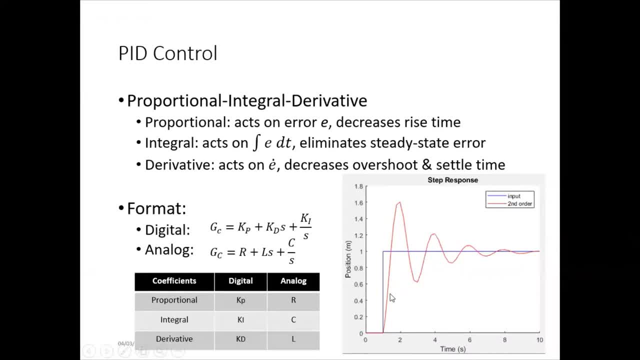 say: this is a step response for a second order system. The blue is the input, so this is where you want your system to be, And then the second order. the red curve is where the system actually is. So the goal would be in this case: let's position on this axis, but you can use it to 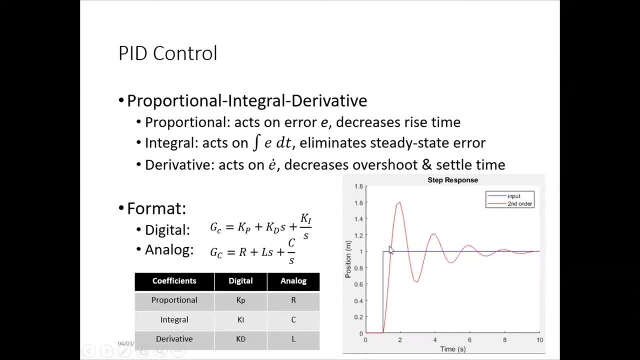 illustrate whatever So say. this is desired temperature and the goal would be to drive the temperature to this certain value. So since the proportional term acts on the error decreasing the rise time, then the farther away the actual system is from the desired, the harder it will. 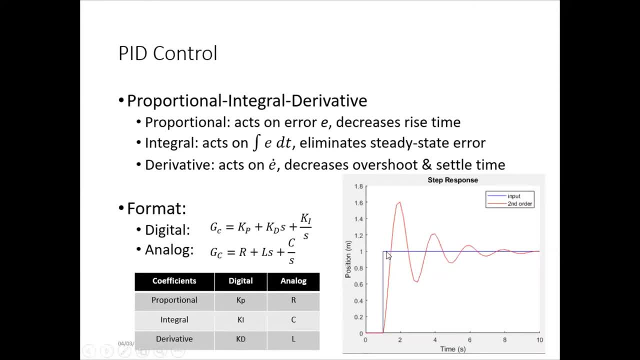 try to pull the system. So this part right here is rise time. So with a high KP there is less difference between start of signal and time that the system reaches it. With a low KP this would be a little bit stretched out And PID control can use any combination of these. So you